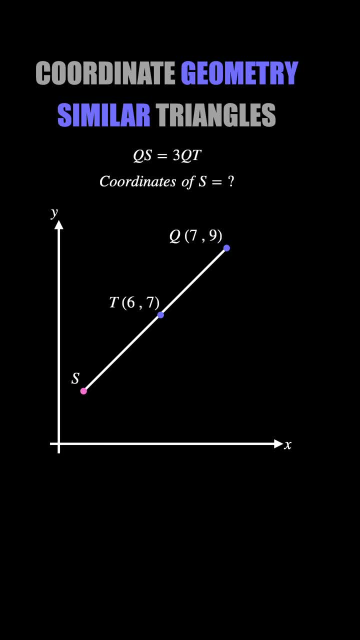 Given that t lies on the line qs and qs equal to 3 times of qt, find the coordinates of s. We'll begin by drawing the triangle with q and t. The horizontal distance between q and t can be found by the difference between their x coordinates 7 and 6. Then we multiply by 3 to get the horizontal. 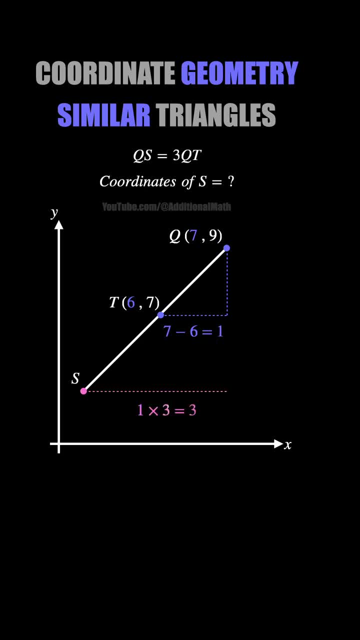 distance of q and s to be 3.. The vertical distance between q and t can also be found by the difference between their y coordinates 9 and 7.. Similarly, we multiply by 3 to get the vertical distance between q and s to be 6.. From q, the coordinates of s is on the left, so we'll subtract the 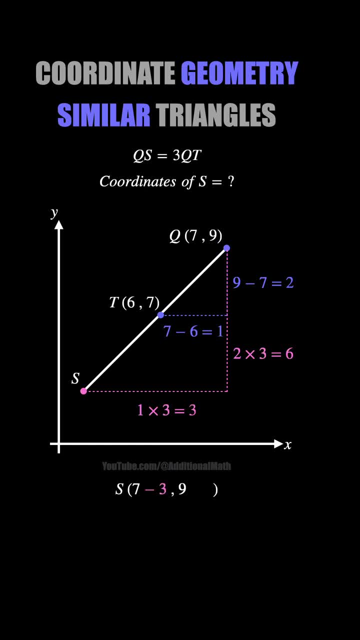 horizontal distance of 3 from the x coordinates, And since s lies below q, we now subtract the vertical distance of 6 from the y coordinates, And that's the answer. 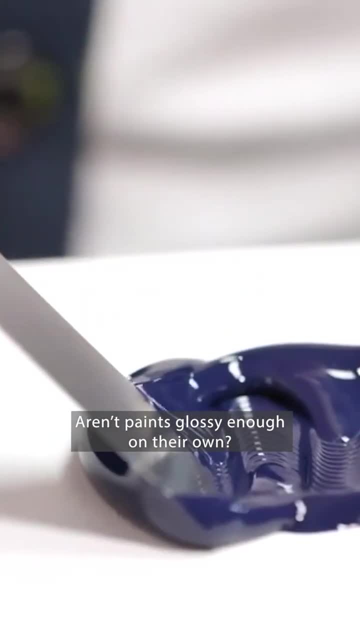 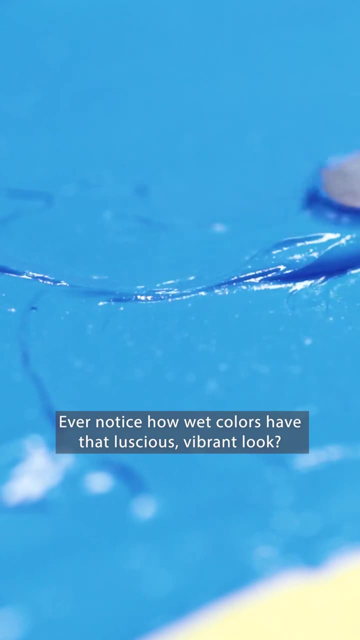 What's the deal with gloss painting mediums? Aren't paints glossy enough on their own? The truth is, gloss mediums do a lot more than just make colors shiny. Ever notice how wet colors have that luscious, vibrant look? Gloss mediums are a game changer. 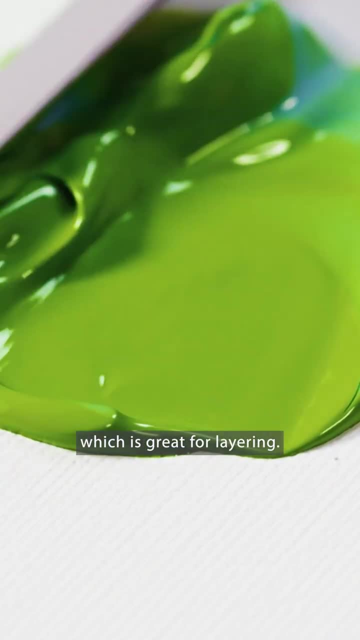 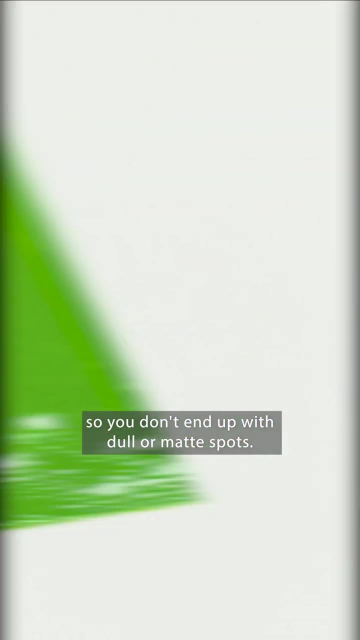 for keeping colors just as vivid as when you first mix them, which is great for layering. Gloss mediums also help even out the shine across the surface of paintings, so you don't end up with dull or matte spots. It's all about making sure people see your amazing artwork. 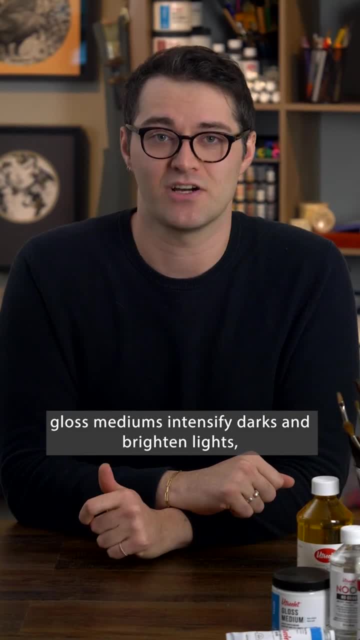 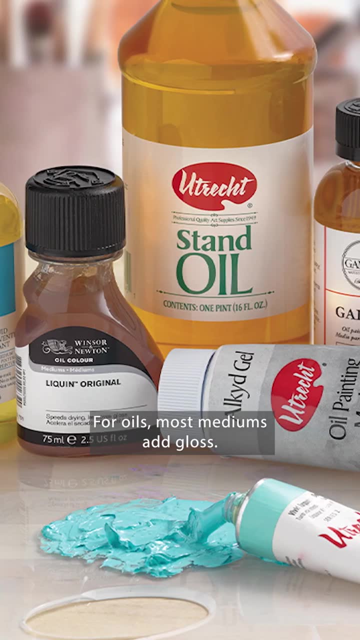 not just the paint- And get this. gloss. mediums intensify darks and brighten lights, so dark colors get deeper and lighter. mixtures are more resistant to staining when you glaze over them. For oils, most mediums add gloss, but when it comes to acrylics, 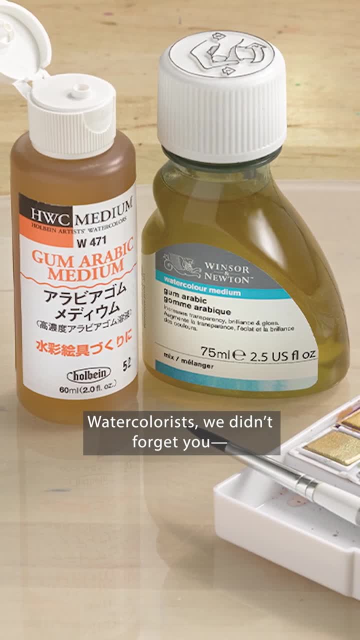 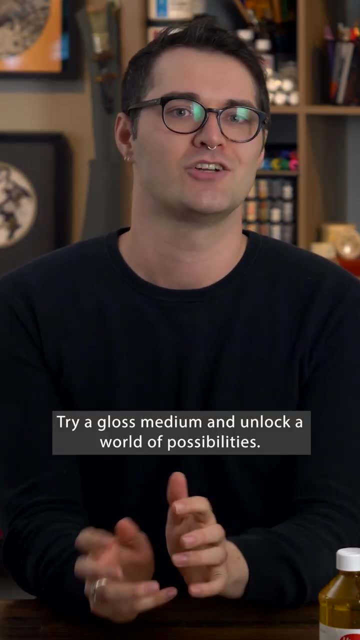 look for mediums with gloss finish on the label. Watercolorists, we didn't forget about you. Try gum, arabic or watercolor medium for that glossy depth. If you're feeling stuck with your color straight from the tube, try a gloss medium.